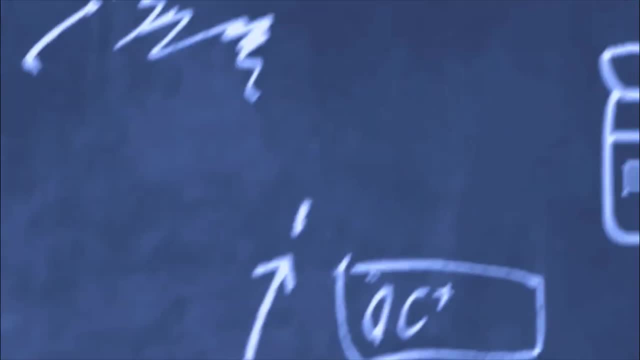 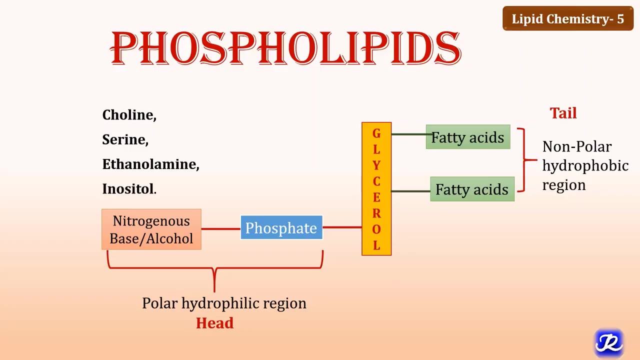 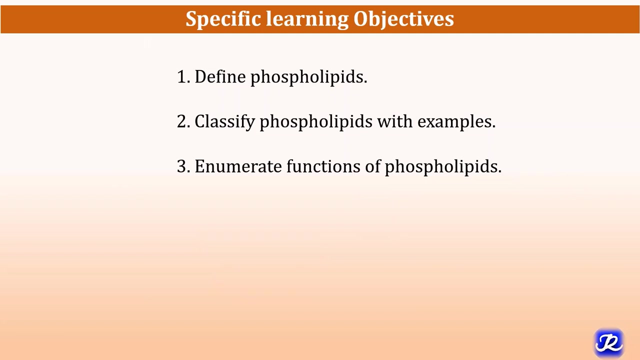 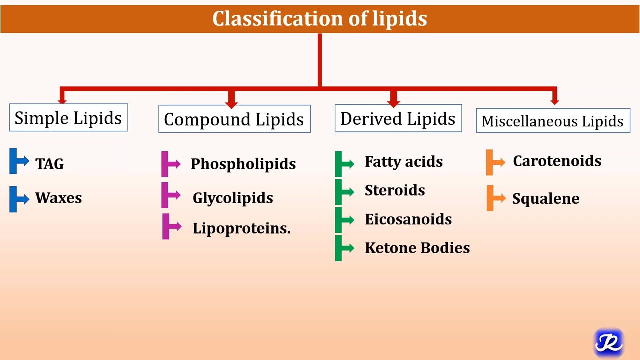 Hello everyone. today we are going to learn about phospholipids. At the end of this session, you should be able to define phospholipids, classify them with examples and enumerate functions of phospholipids. Before going into details of phospholipids, let's first understand what are lipids. 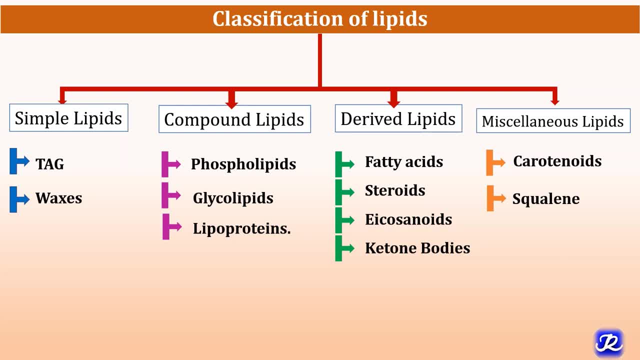 Lipids are the organic substances which are relatively insoluble in water, but they are soluble in non-polar organic solvents like alcohol, ether, benzene, chloroform, etc. They are actually or potentially related to fatty acids and utilized by the living cells. 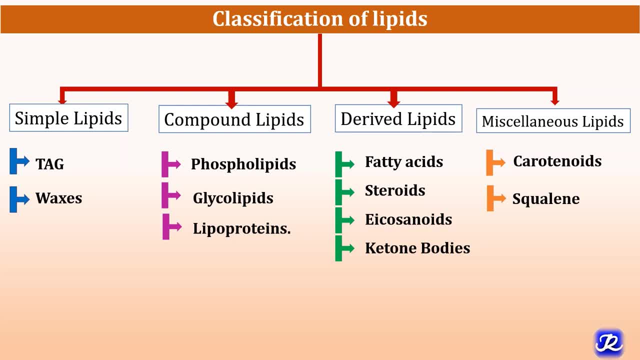 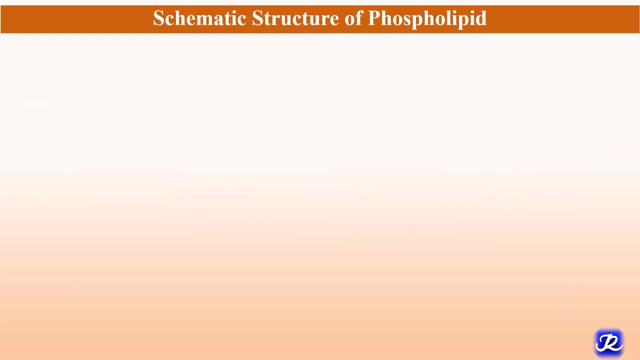 Lipids are classified into simple lipids, compound lipids, derived lipids and miscellaneous lipids. Phospholipids are compound lipids which are made up of fatty acids, alcohol, phosphoric acid and nitrogenous base In the structure of phospholipid. 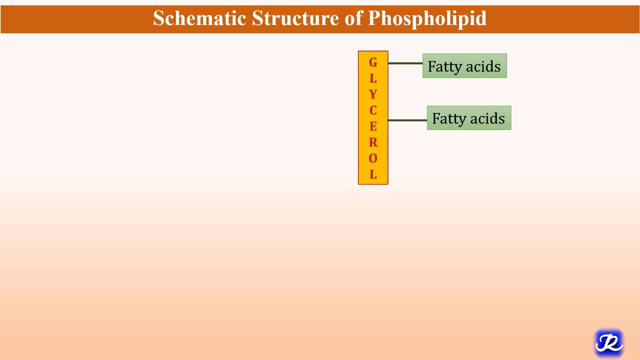 two fatty acids are attached to glycerol. The carboxyl group of two fatty acids are attached to hydroxyl group of glycerol at C1 and C2 position, and hydroxyl group at C3 position is attached to phosphate, which is further attached to nitrogenous base. 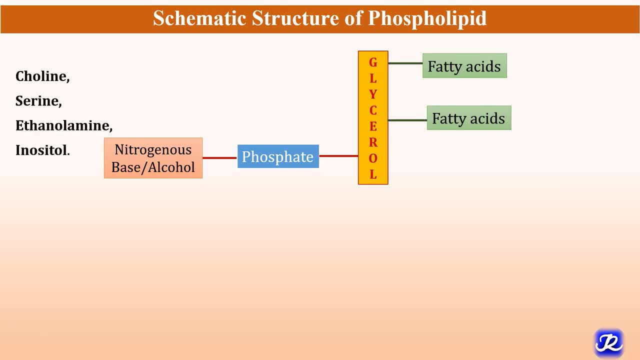 Soy sauce or glycolic acid, is attached to hydrophobic acid, and this group is later connected with the glycemic acid, which is also directly отноlere to phosphore. Phospholipids are made up of lactose. describing the combination between: 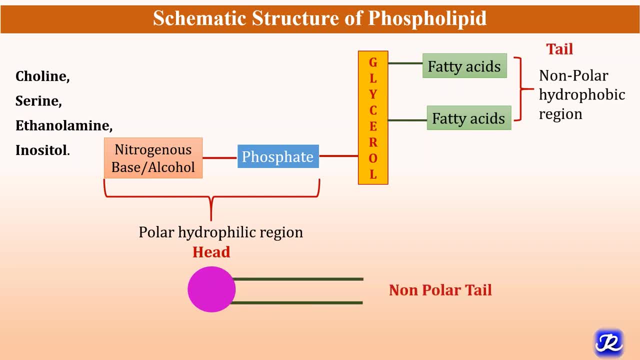 non-nitrogenous and even the anaerobic active compound. X. Symptoms of lunar은 Ver manual of nitrogenous base or alcohol, and this can be chlorine, serine, ethanolomatine, inositol. these nitrogenous base and phosphate together forms a polar hydrophilic region. it is called as head and tail. fatty acid forms a tail, which is nonpolar hydrophobic region, and this polar head and nonpolar tail make phospholipid, a ampebatic molecule which is the important constituent of cell membranes, which are not just our ass. 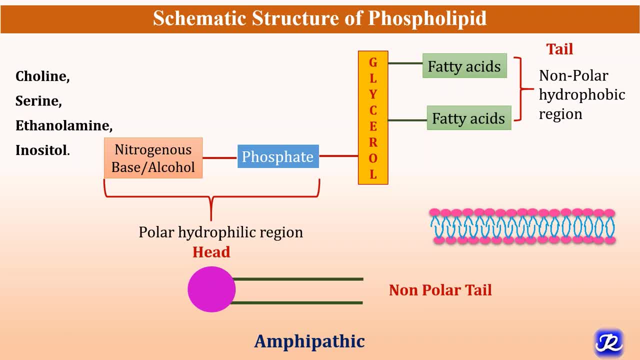 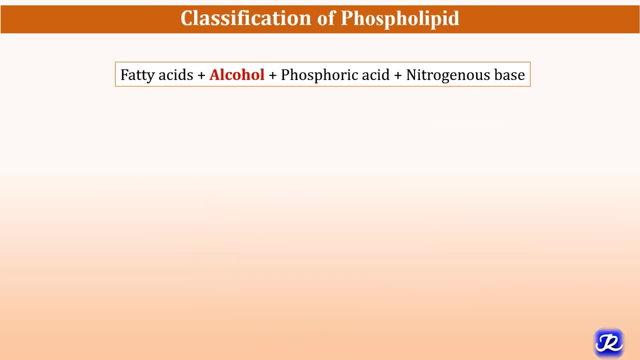 brain, which is a lipid bilayer where head faces towards the aqueous medium and tail faces towards each other, as they are hydrophobic. Classification of phospholipid is based on the type of alcohol present in it. If the alcohol is glycerol, they are called as glycerophospholipid. 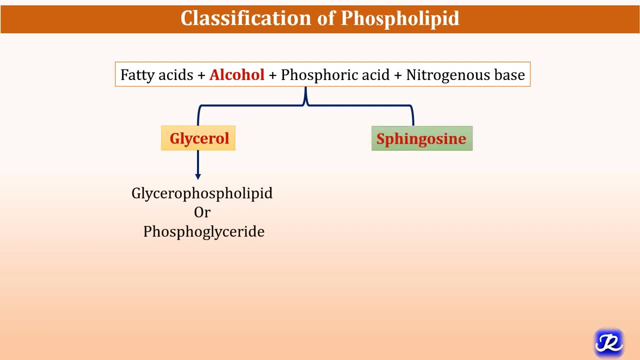 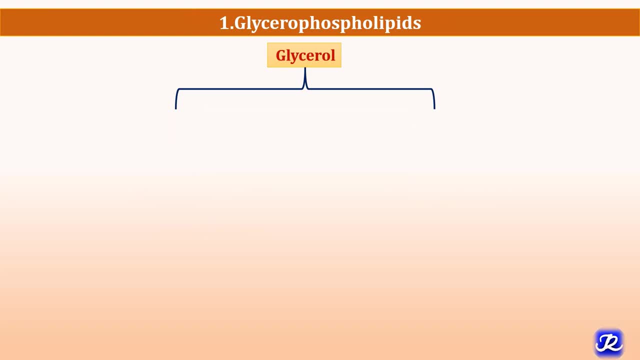 or phosphoglyceride. If the alcohol present in phospholipid is sphingosine, they are called as sphingophospholipids, The glycerophospholipids, which contains glycerol as alcohol. they are further classified based on the presence or absence of nitrogenous base, that is, with nitrogenous base. 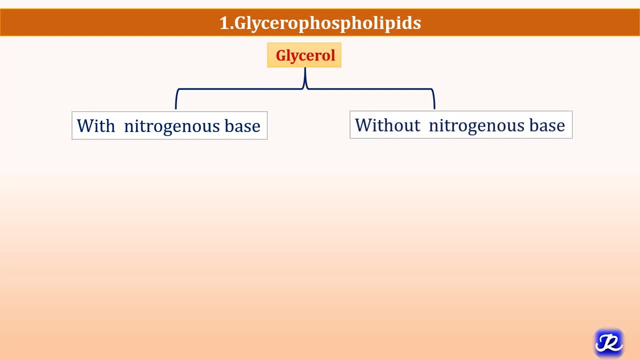 and without nitrogenous base. The example of glycerophospholipids with nitrogenous base are lecithin, which is also called as phosphatidylcholine, cephalins, phosphatidylethanolamines, phosphatidylserine and plasmalogen. 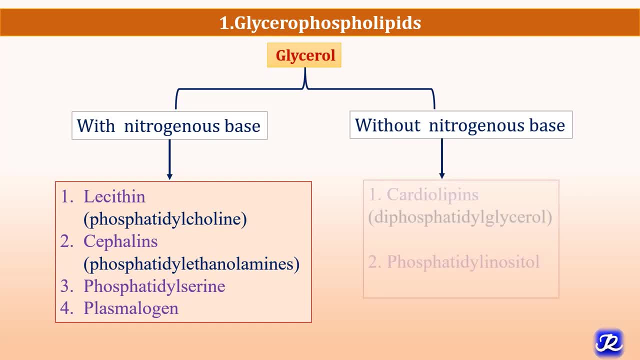 Glycerophospholipids without nitrogenous base are kydolipins also called as diphosphatidylglycerol and phosphatidylinositol. Before discussing the examples of phospholipids, let's understand what is phosphatidic acid. 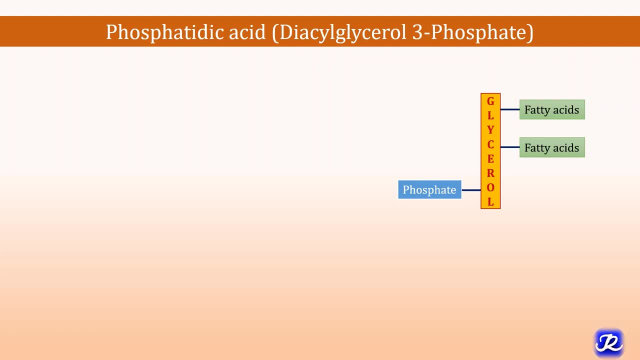 It is a diacylglycerol 3-phosphate. Here you can see that two fatty acids are attached to glycerol and at the C3 position phosphate group is attached. There is no nitrogenous base or alcohol attached to the phosphate group, So this is a phosphatidic acid and it is the 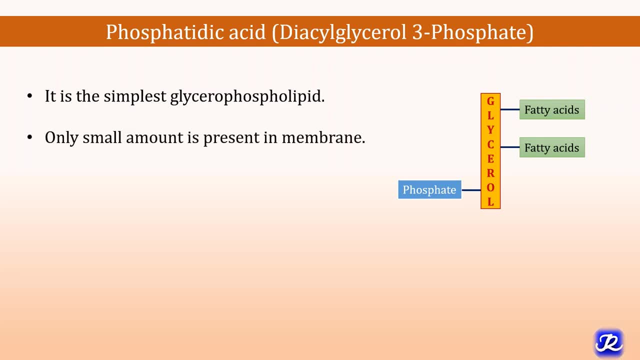 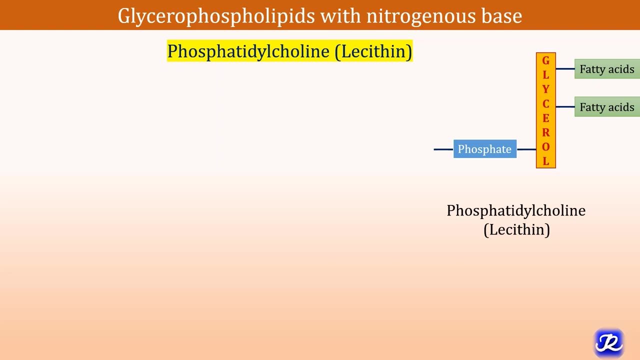 simplest glycerophospholipid. Only small amount is present in the membrane, and this phosphatidic acid is the key intermediate in the synthesis of other glycerophospholipids. The first glycerophospholipid with nitrogenous base is phosphatidylcholine, which is also called as lecithin. The nitrogenous base is: 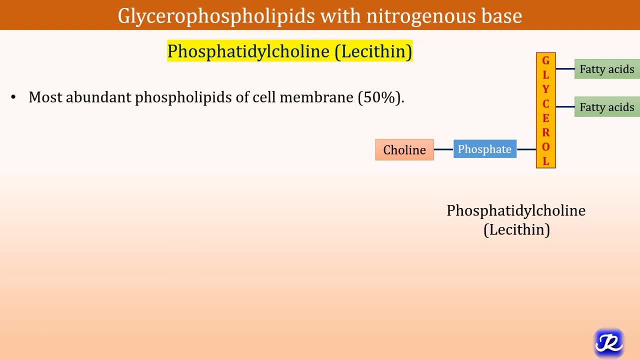 choline. here It is the most abundant phospholipids of cell membrane. It is about 50% of all the phospholipids which are present in the cell membrane. It is also involved in the formation of lipoproteins, as well as acidification of cholesterol. Choline are largely stored as phosphatidylcholine and 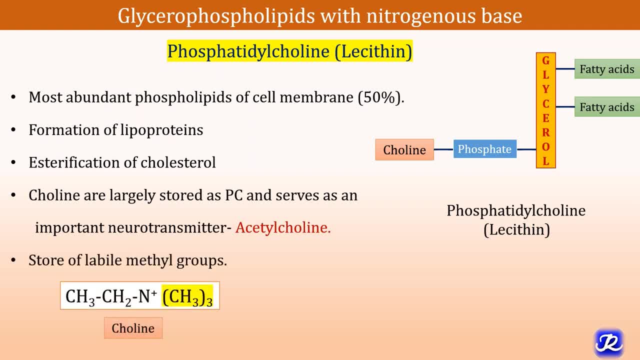 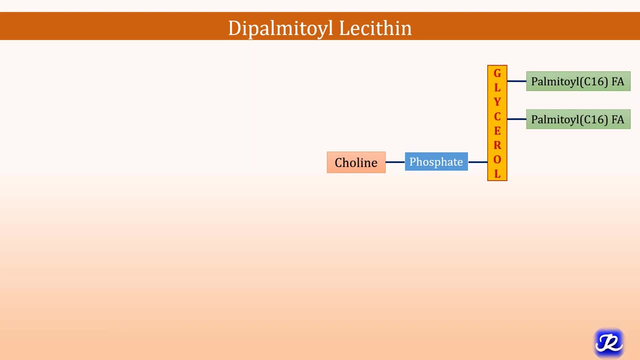 serves as an important neurotransmitter. that is acetylcholine. It is a storage of labile methyl groups which are involved in the transmethylation reactions. When two fatty acids attach to glycerol are palmitoyl fatty acids, the lecithin becomes dipalmitoyl lecithin. 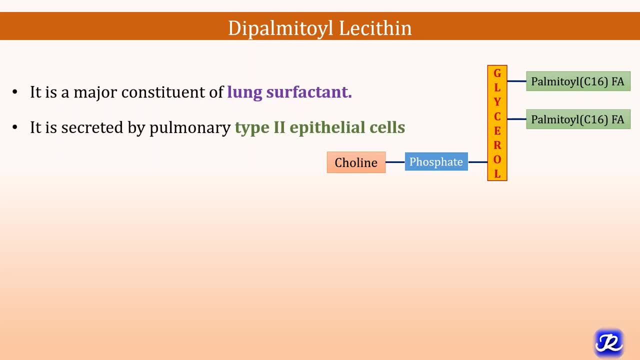 It is the major constituent of lung surfactant, which is secreted by pulmonary type II epithelial cells. The surfactant reduces surface tension in the alveoli and prevents adhesion of inner surfaces of the lungs, which in turn prevents alveolar collapse. Absence of surfactant results in respiratory distress syndrome. 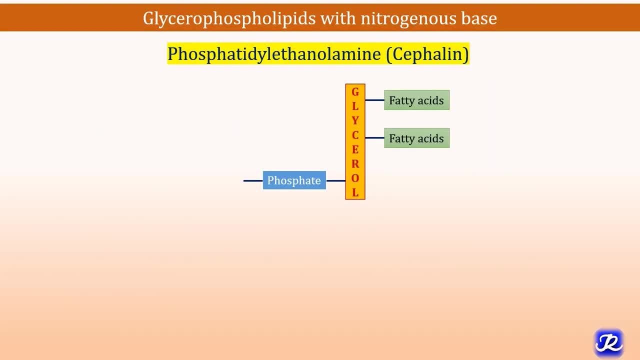 in premature infants. The second glycerophospholipid with nitrogenous base is phosphatidylethanolamine, which is also called as cephaline, and in the structure, ethanolamine is attached to phosphate Thromboplastine, which is also called a coagulation factor III, which is required for clotting. 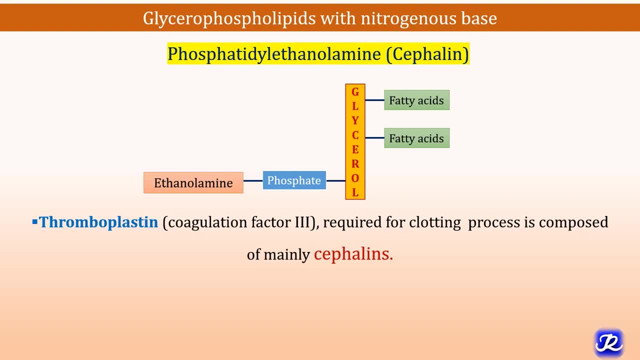 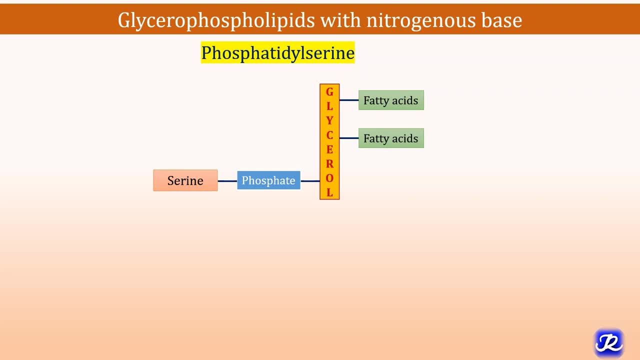 process is composed of mainly cephalines. The third glycerophospholipid with nitrogenous base is phosphatidylserine, where the nitrogenous base attached to phosphate is serine, And this is the 10% of phospholipids in mammals. 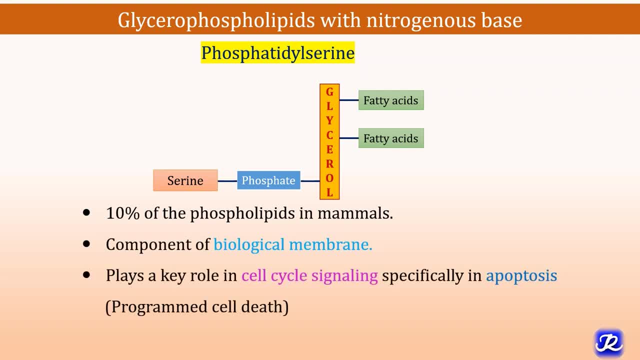 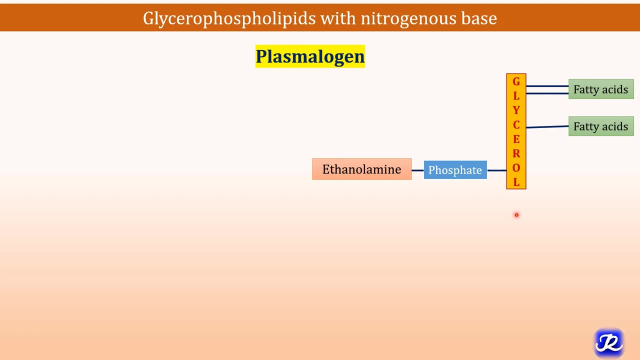 It is the component of biological membrane and it plays a key role in cell cycle signaling, specifically in apoptosis, that is, programmed cell death. Plasmalogen is a glycerophospholipid with nitrogenous base. The structure is similar to cephaline, that is, phosphatidylethanolamine. 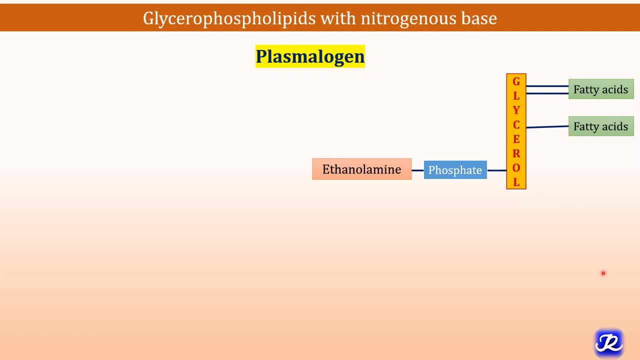 Only difference is that the fatty acid is attached with the ether linkage. There are three glycerophospholipids: The first, glycerophospholipid with nitrogenous base. The second, glycerophospholipid with nitrogenous base. 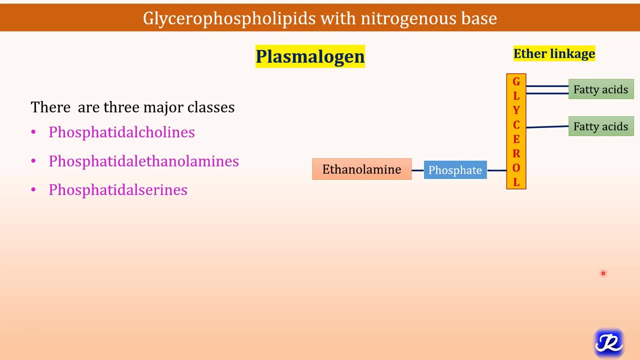 The third, glycerophospholipid with nitrogenous base And the fourth, glycerophospholipid with nitrogenous base. These are the three major classes, depending upon the base which is attached. These are phosphatidylcholine, phosphatidylethanolamines and phosphatidylserine. 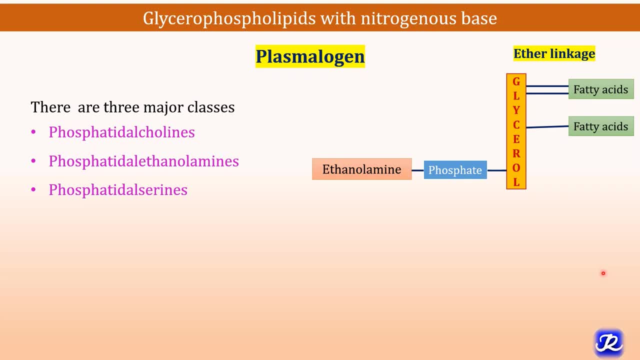 These are found in myelin and cardiac muscle. Platelet activating factor, that is, PAF, is a plasmalogen and involved in platelet aggregation and degranulation, and it may have protective effect against reactive oxygen species. Now let's see the glycerophospholipids. without glycerophospholipid? 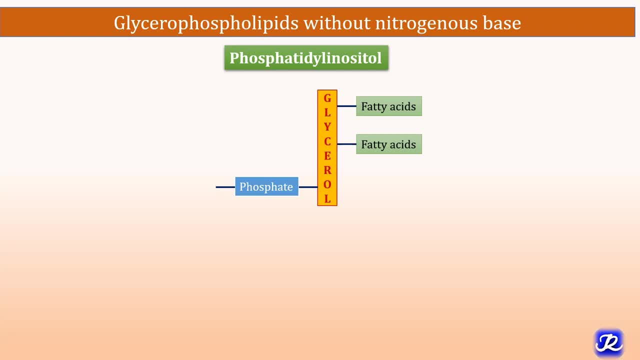 nitrogenous base, and the example is phosphatidyl inositol, where the phosphate group is attached to myoinositol and that act as a second messenger for the action of hormones like oxytocin and vasopressin. The second glycerophospholipid without nitrogenous base is cardiolipin, in which you can 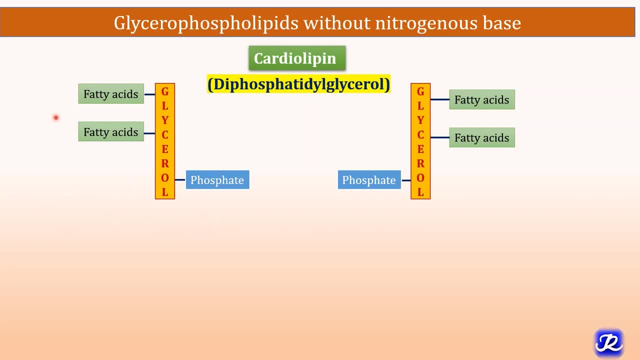 see two phosphatidic acid. This is the one phosphatidic acid and this is the second phosphatidic acid. They are linked together by glycerol so it becomes cardiolipin. It is the major lipid of mitochondrial membrane. It is necessary for the electron transport process and this is the only. 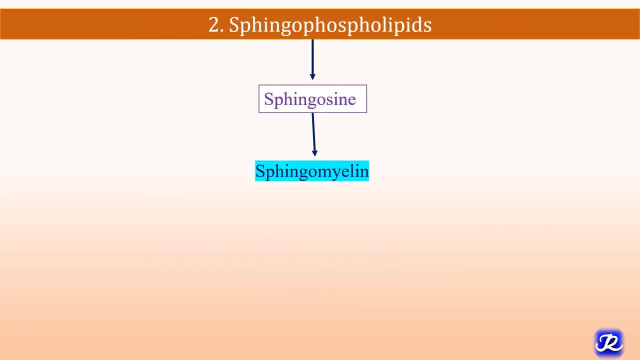 phospholipid, which is antigenic in nature. The second class of phospholipid is sphingophospholipid, which is made up of alcohol, sphingosine, and the example is sphingomyelin. Sphingosine is derived. 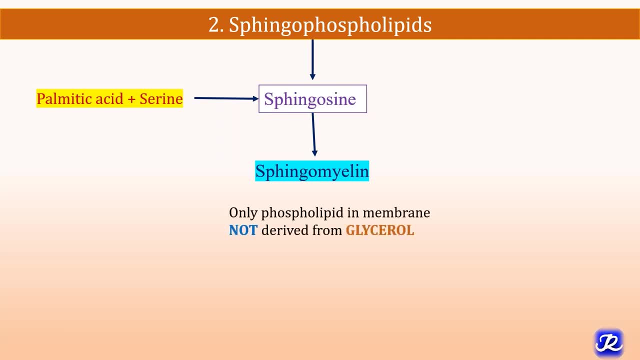 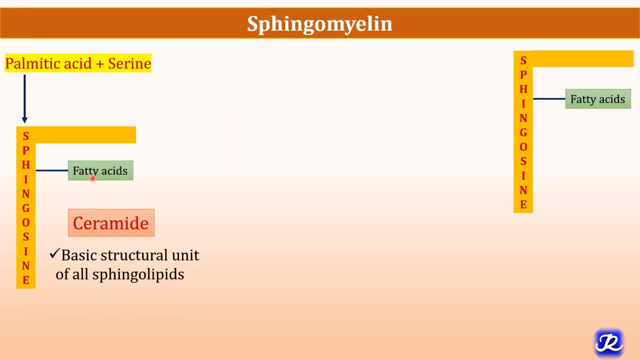 from palmitic acid and serine, And sphingomyelin is the only phospholipid in membrane which is not derived from glycerol. When sphingosine is attached to fatty acid, it becomes ceramide, So ceramide is sphingosine. 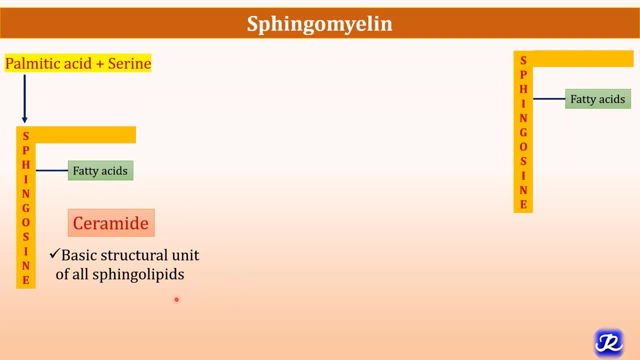 plus fatty acid and it forms a basic structural unit of all sphingolipids. So when the sphingosine is attached to fatty acid and further it is attached to phosphate group and cooling it becomes sphingomyelin. So sphingomyelin is composed of ceramide plus phosphate plus 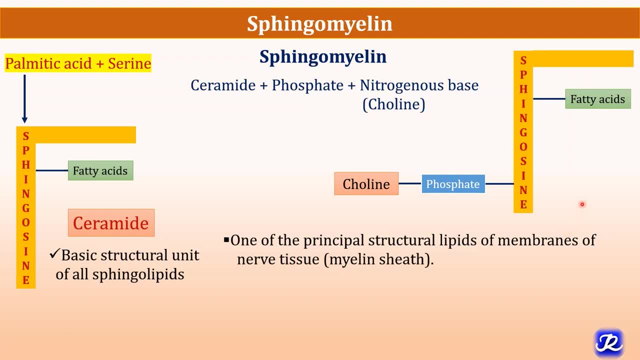 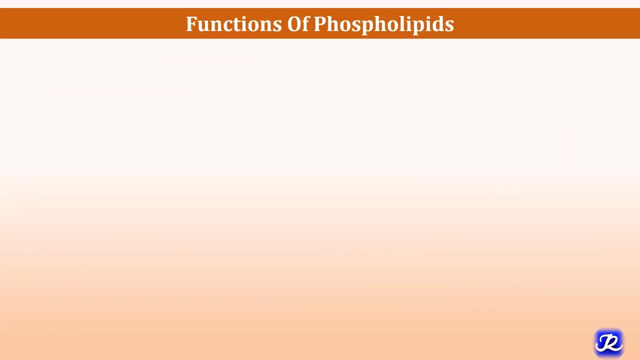 nitrogenous base And it is one of the principal structural lipids of membranes of nerve tissue, Act as a electrical insulator around nerve fibers and play a key role in cell signaling and apoptosis. So far we have seen the phospholipids, their classification and important functions. Now let's enumerate all the. 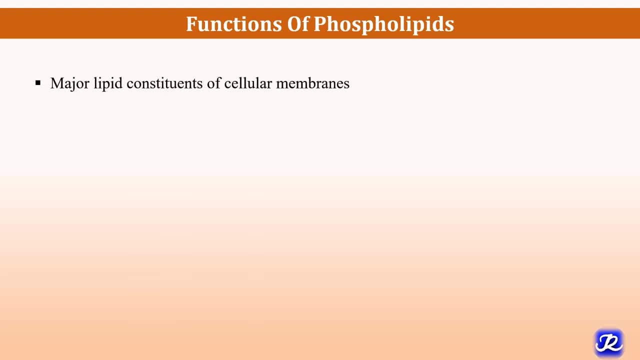 functions together. Phospholipids are the major lipid constituent of cellular membranes. They regulate permeability Of membranes and activation of some membrane bound enzymes. They are good emulsifying agents and help in intestinal absorption of lipids. They are the constituent of lipoproteins and 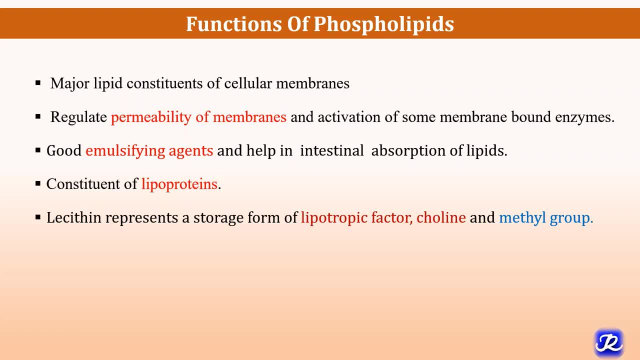 lecithin represents a storage form of lipotropic factor, choline and methyl group. Lipotropic factor is a factor which prevents deposition of triacylglycerol in liver, that is fatty liver. Lecithin acts as lung surfactant, which prevents alveolar colon. So lecithin acts. 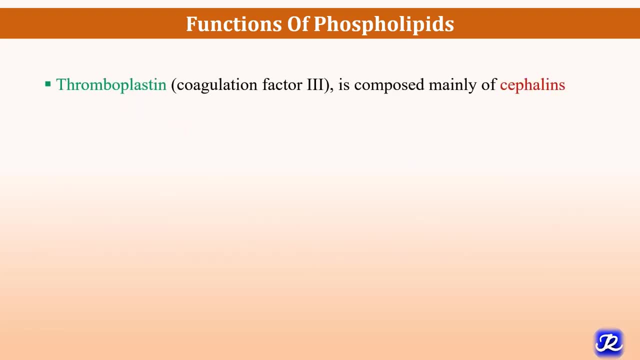 as a lipoprotein which prevents prolapse- Thromboplastin, that is, coagulation factor 3. it is composed mainly of cephalins. Phosphatidyl inositol is a second messenger for hormones like oxytocin and.